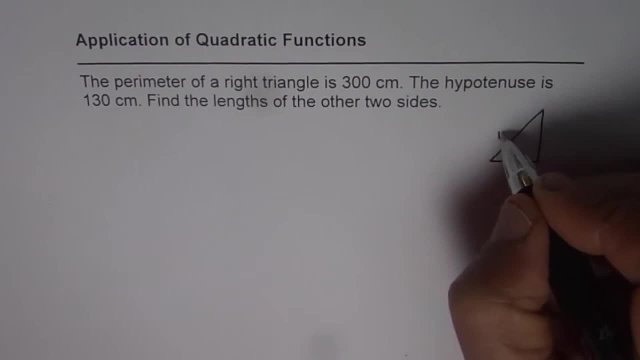 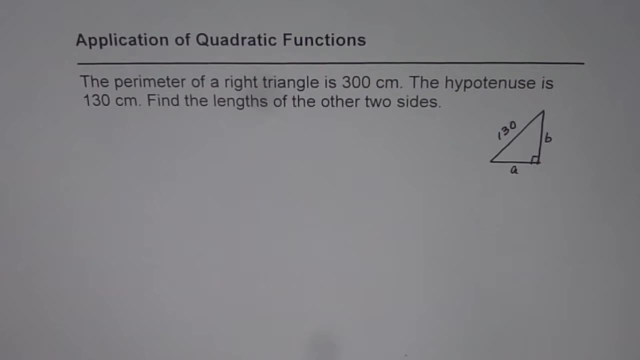 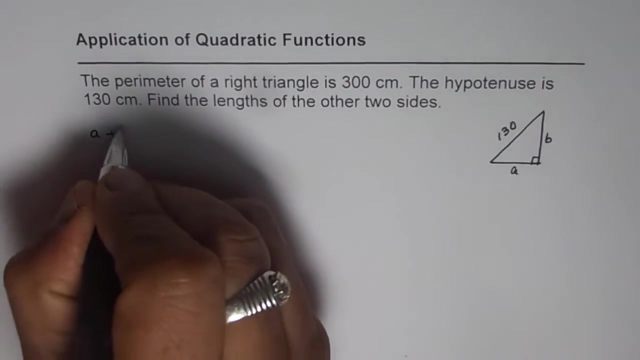 triangle. we are given the hypotenuse as 130 centimeters and the other two sides let them be a and b. Now the relations, we can write two of them. One of them is the perimeter. So we have a plus b plus 130, which is the hypotenuse is equal to 300. So that is one. 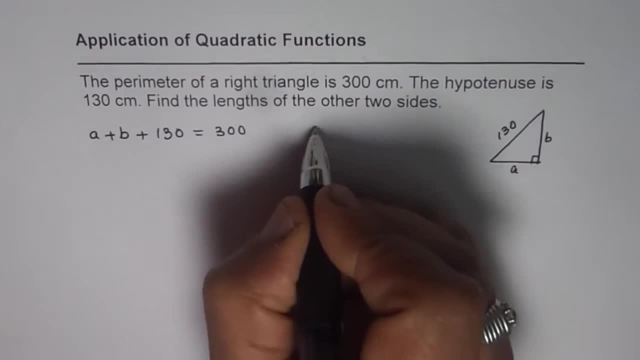 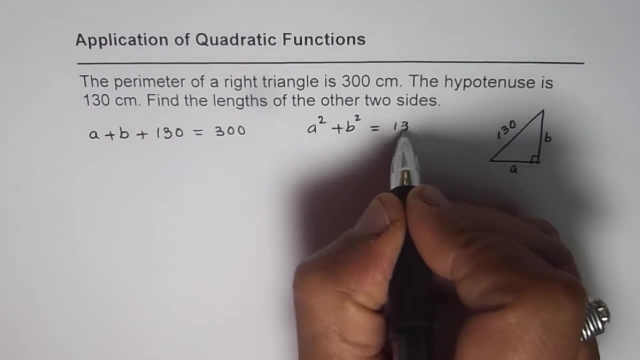 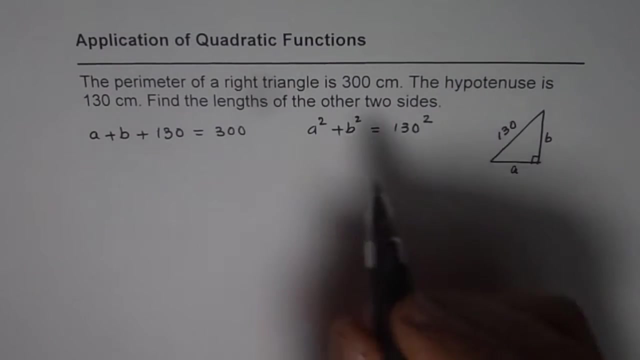 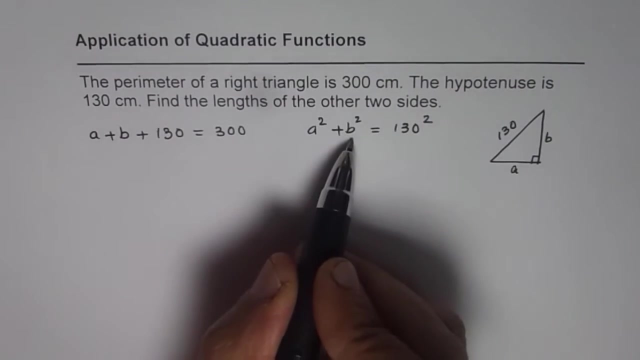 relation, The other one we get from the Pythagorean theorem, which is: a square plus b square is equal to 130 square. So these are the two relations. There are two variables, a and b, which we can always find. So from here we can write what the value of a is in terms of b And then use this equation to 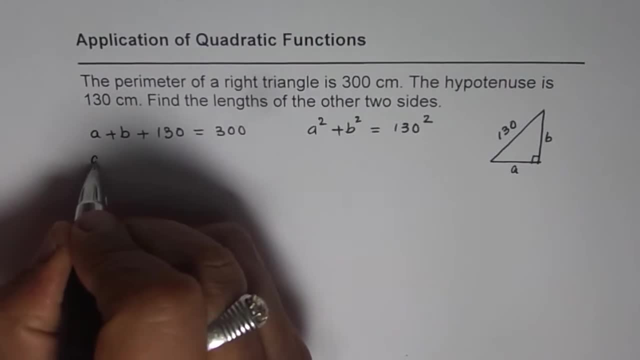 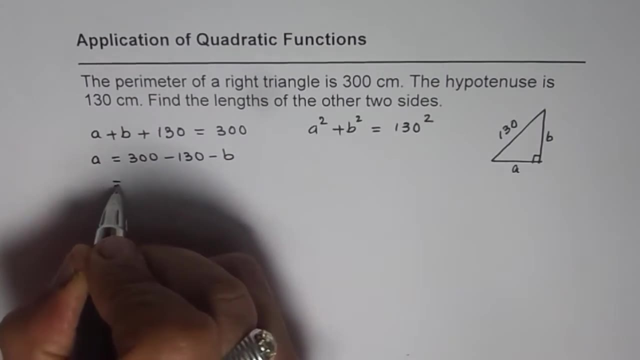 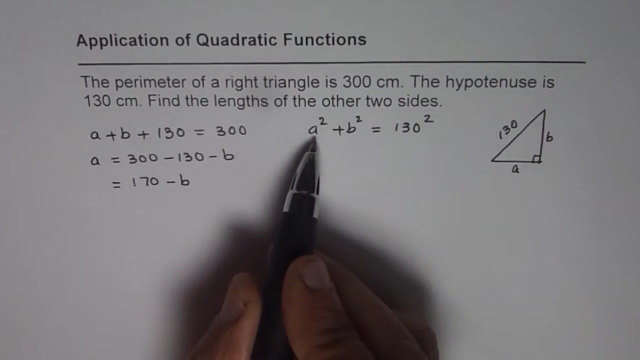 find the variable b. So we can write: a is equal to 300 minus 130 minus b, and that is 170 minus b. So that is the value of a. Now this equation. let us substitute this value of a in the equation and find b. so what we get here is: 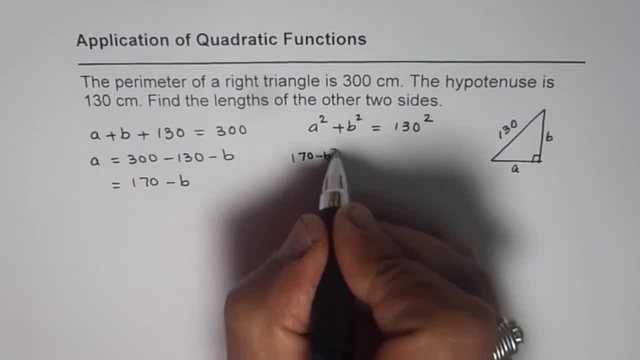 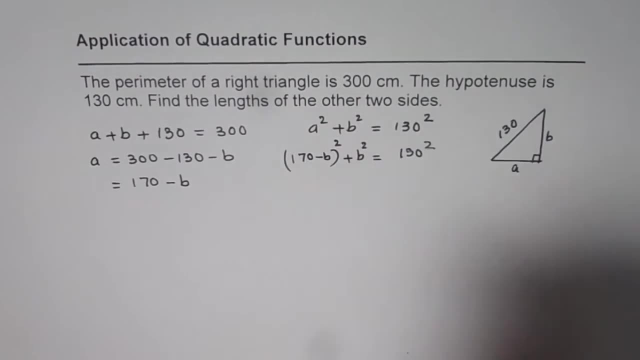 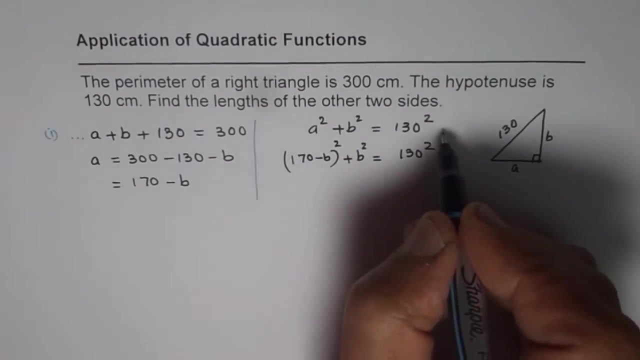 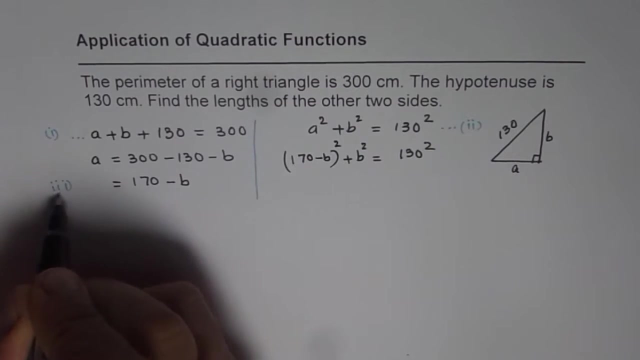 170 minus b whole square plus b square is equals to 130 square, correct? i hope you understand that part. so we began with two equations. let's say that is equation number one. this is equation number two. from equation number one we found what a is in terms of b, so we substitute this value here. 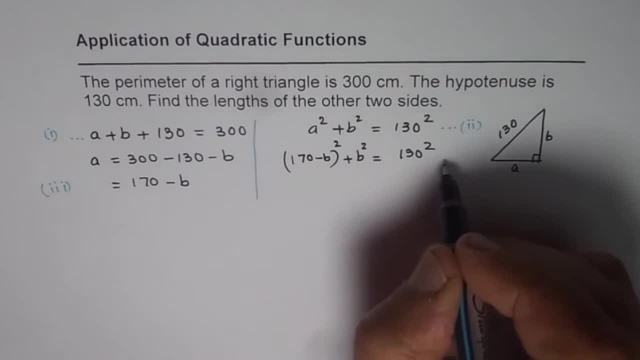 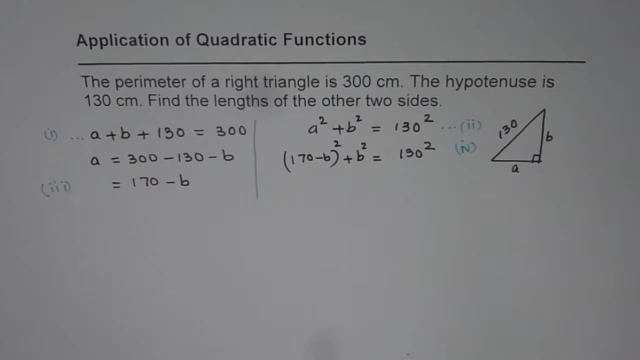 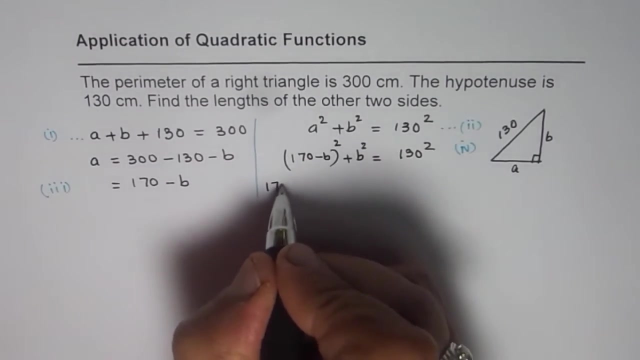 in this equation, in equation two, and so we have a equation- let me call this equation four- in one variable. now we'll can solve for b from this particular equation, right, so let us expand this. we got 170 square. let me write first: 170 square minus two times. 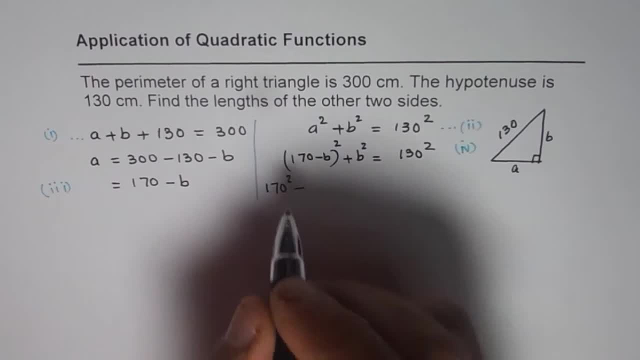 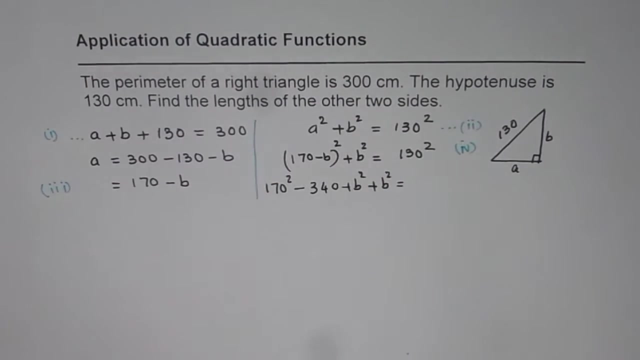 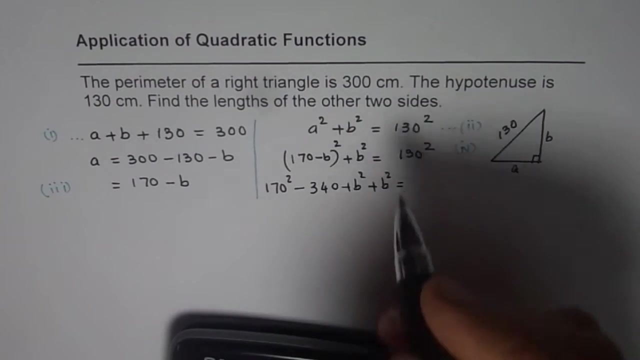 b 170 times b. so two times 170 will be zero. two times seven is fourteen four one three forty plus b square plus b square equals to 130 square. okay, we can use calculator 16900. anyway. we should use calculator. so we have 169, 13 square is 169 and we get 00. so let us further simply. 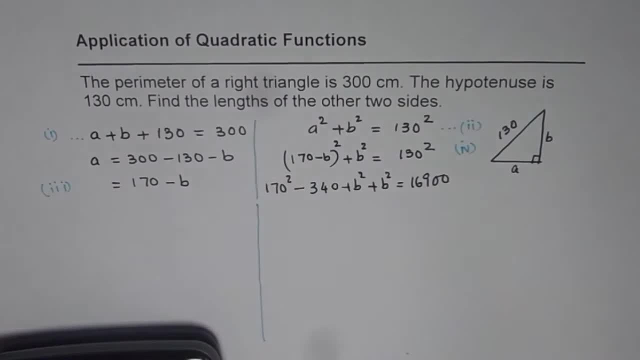 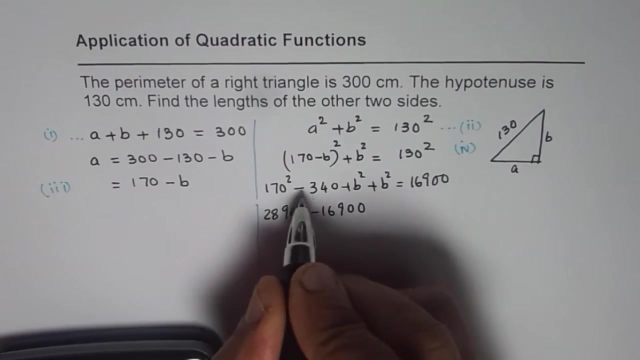 and find the value of b from this equation: 170 square is how much? 170 square is equal to 28900. so we have two, eight, nine zero, zero. we're bringing 169 also on this side, minus 16900, minus 340, 340 b. 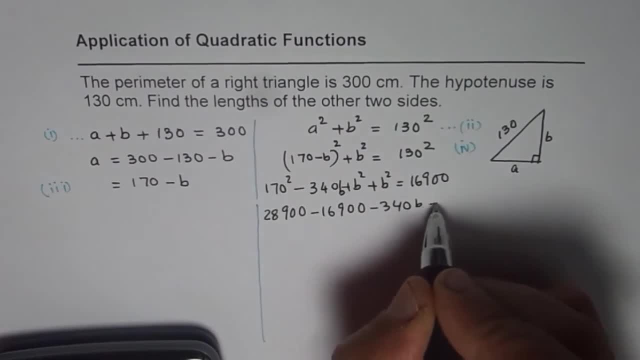 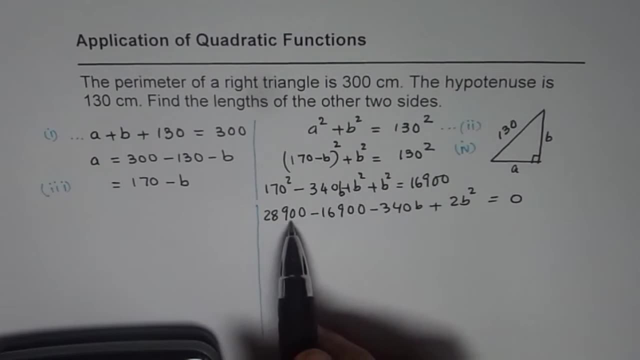 to ab right. minus 340 b plus two b square equals to zero. that's what we have. so let's do this: 28900 minus 16900 is how much is equals to one twenty thousand. so we'll rearrange right this equation as two b square minus 340 b plus 129. 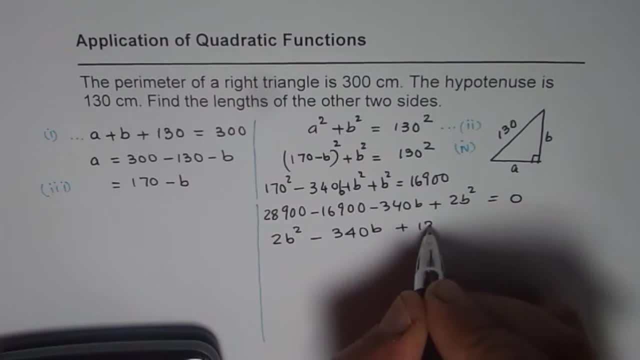 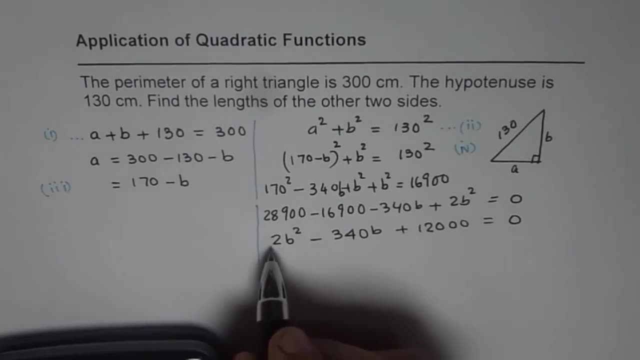 b plus 120. so we'll rearrange. write this equation as two: b squared minus 340b plus 120, b squared minus 3400 plus 120000, 100, 12,000 equals to 0.. So that is a quadratic equation. Let's factor out 2.. We can write this: 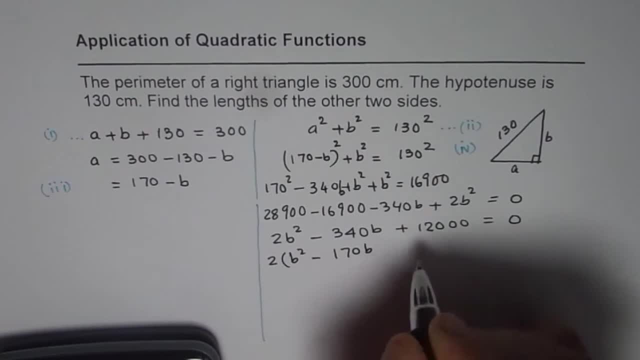 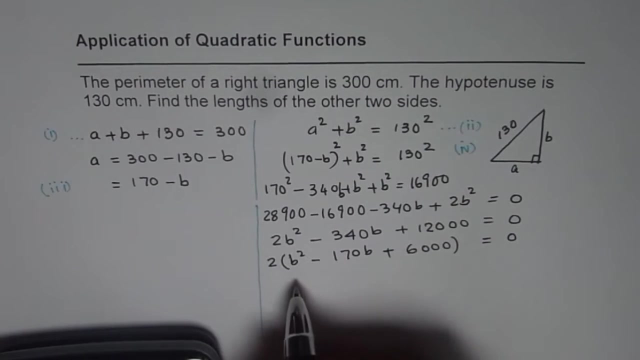 as b. square minus 170, b plus divide by 2 will give us 6,000.. 6,000 equals to 0.. Now to solve this we can use quadratic formula. So that is easy way. So we can get value of b as minus of b. 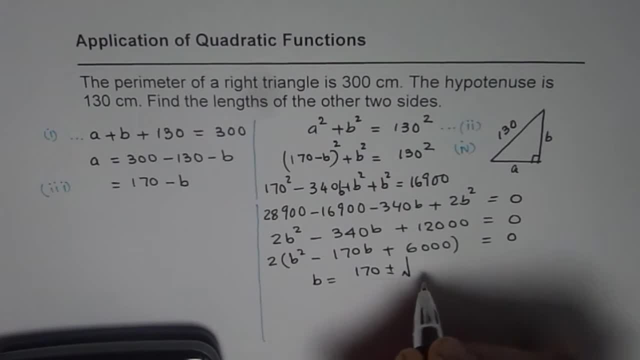 which is 170 plus or minus square root. square of this square of 170 minus 4 times a is 1,. c is 6,000. square root divided by 2 times coefficient of a, which is b square, is 1,, 2 times 1.. So that 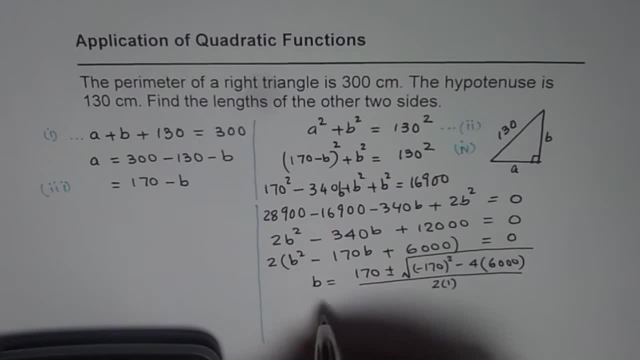 is what we get. So let's use calculator to find how much is this equal to. So we have 170 plus and minus. So we have 170 square minus 4 times. that means 24,000, 24, 1, 2, 3, 0s. 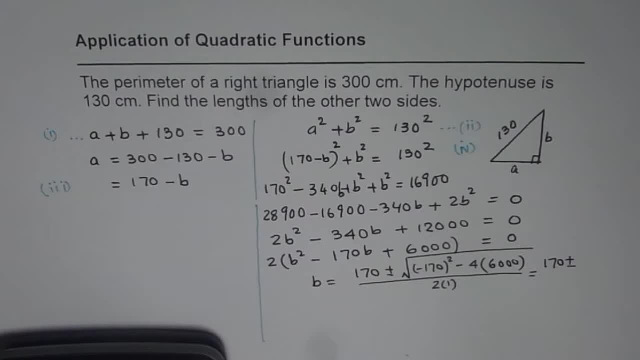 4,900. square root of 4,900 is, you know, 7, square root 10.. So we add the number of stax at the derivates, The number of stax in 7,. let me just write this. and now we have 740,, 20,, now 950, and 10,. this and 12, and 12,, so going on and so. 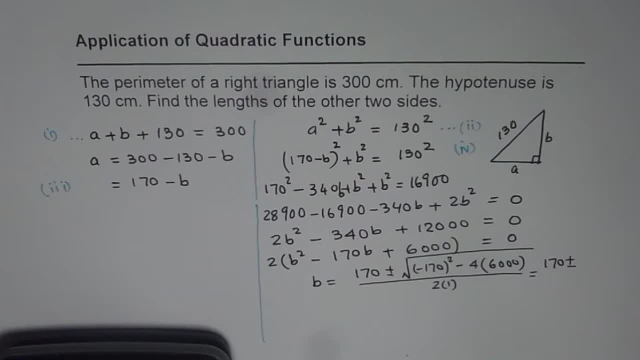 forth, Because 1,, 2,, 3,, 4, I know 1, 2,, 3,, 4 and so on- 1,, 2,, 3, 4.. So 1,, 2,, 3,, 3,, 4, 4 and 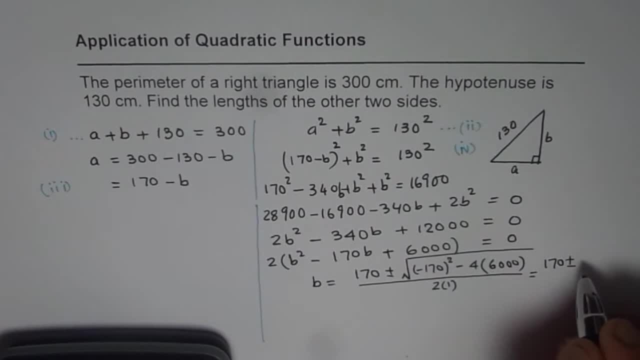 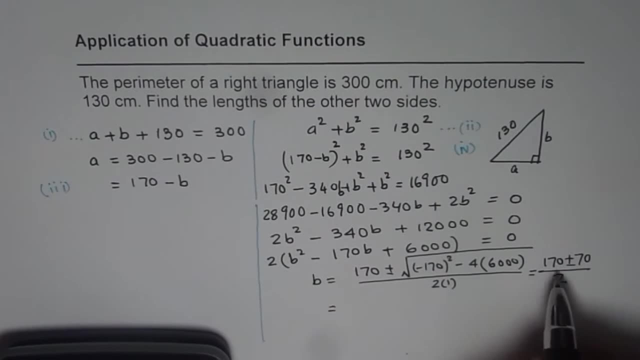 10.. So that is 70.. So we'll write plus minus 70 over 2.. So that gives us two values for B. The two values are 170 plus 70 divided by 2, right? So it is 170 plus 70 divided by 2,, which is 120.. 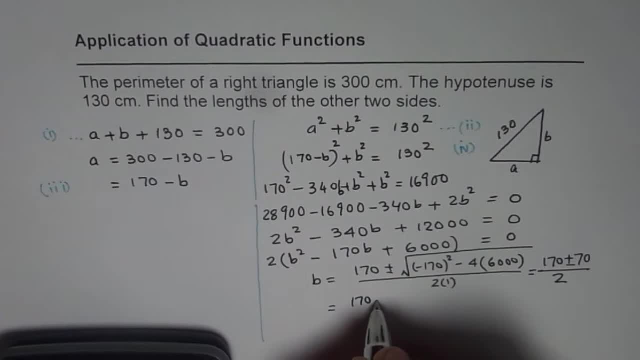 The other one is: so: one is 170 plus 70 divided by 2.. The other one is 170 minus 70 divided by 2, right. So that gives us 100 divided by 2 is 50. And this gives us 200, and I mean 7 times 2 is 14.. And then 1, 3, 240 divided by 2 is 120.. So these are the two values of B which you get right. 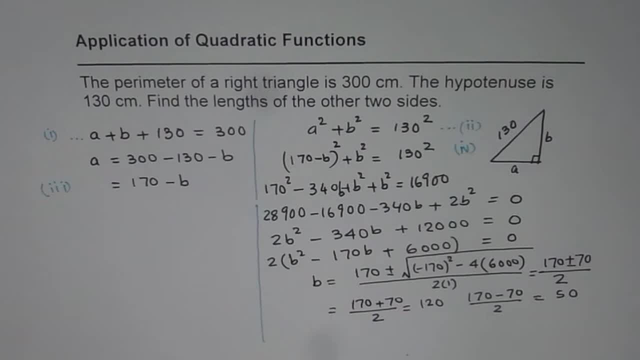 So let us substitute the value of B and find the value of A in our case. So what is A equals to? So what we have here is two different values. One is 50.. The other one is 120.. So we'll substitute both and see which one is the right answer, okay.